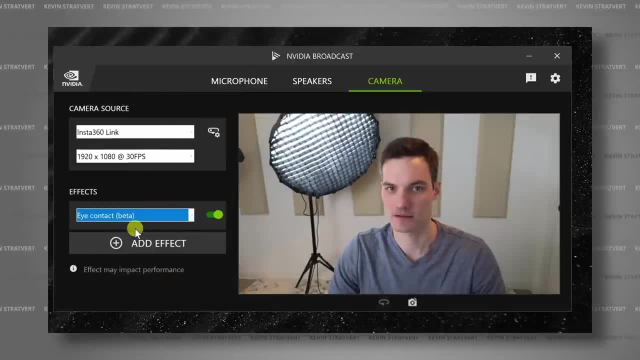 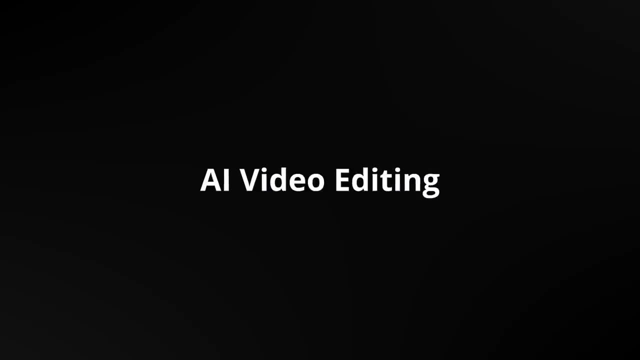 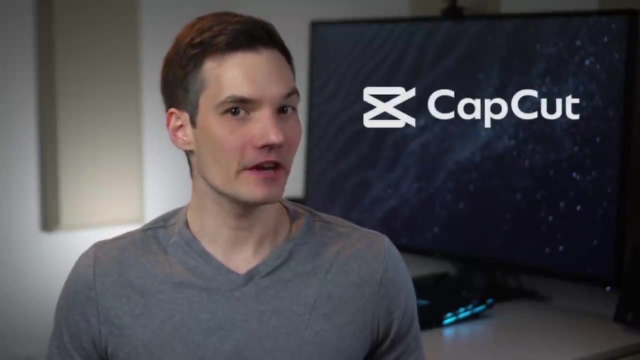 and you could also up-level your video conferencing game. I'm sure at least one of these tools will change the way you work. Let's check these out. First up, I partnered with an amazing AI-powered video editing app called CapCut And let's be honest, video editing can take so 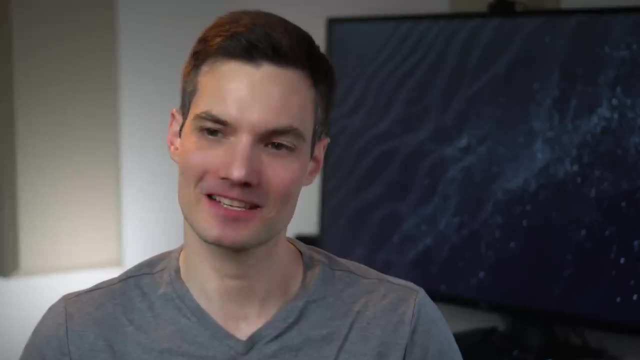 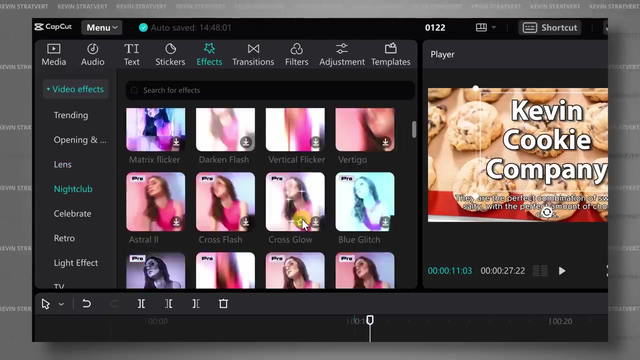 much time, skill and also creativity, and sometimes I just don't have enough of those. CapCut is an extremely powerful and also easy to use video editing app that's free to use. CapCut has all of the core video editing functionality that you would expect. 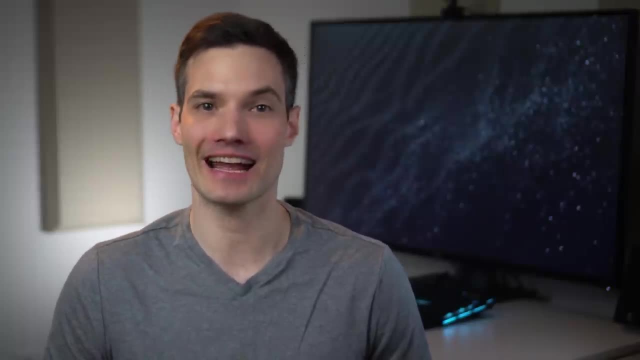 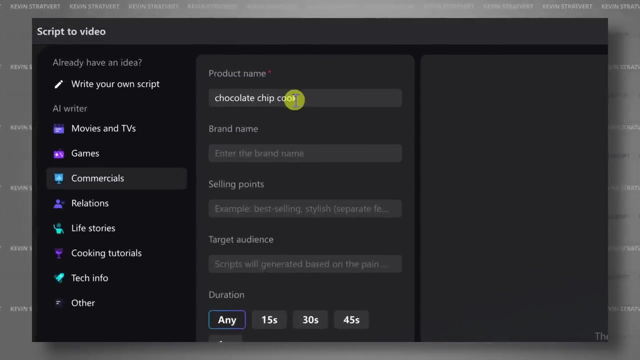 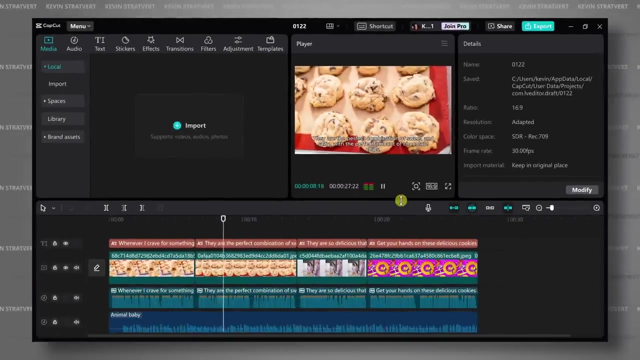 But what makes it stand out from other video editing apps is its extensive use of AI. For example, you can create a video directly with AI. Simply type in some text describing the video that you want, and then CapCut generates a script, a voiceover and even matching images. 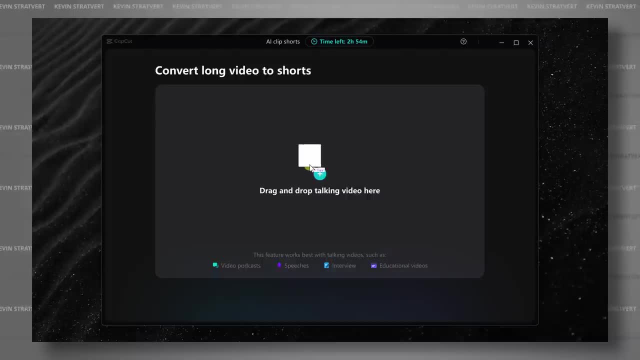 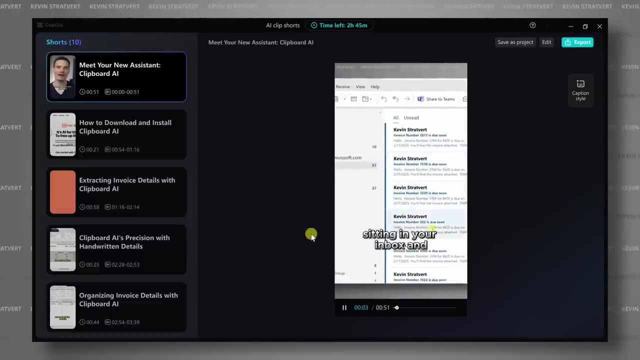 You can also take an existing long-form video and CapCut will automatically convert it into a short that you can upload to, say, TikTok or Instagram. It adjusts the aspect ratio, but it also keeps the subject in frame, and it even adds captions Within the editing experience. 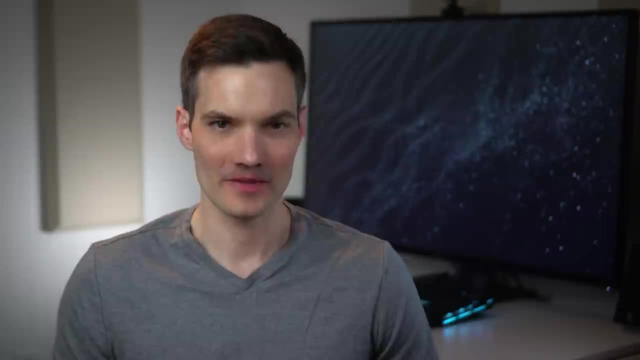 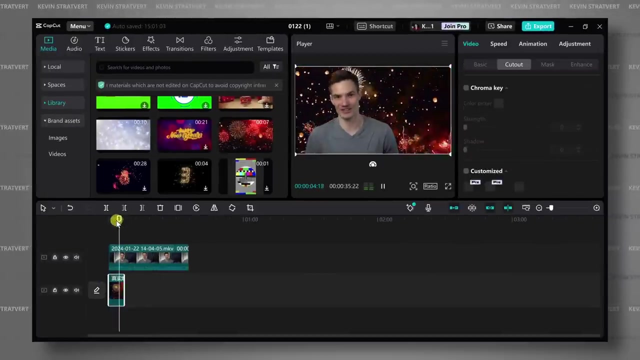 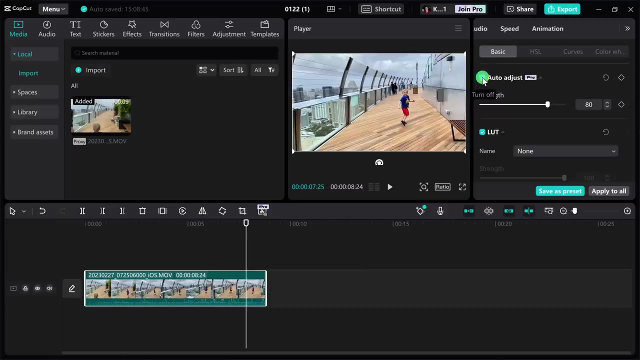 you'll find a wide variety of AI tools. For example, you can remove the background of a video and replace it with any image or color that you want, And you can do all of that without even needing a green screen. You can correct and enhance the color of your video, making it more. 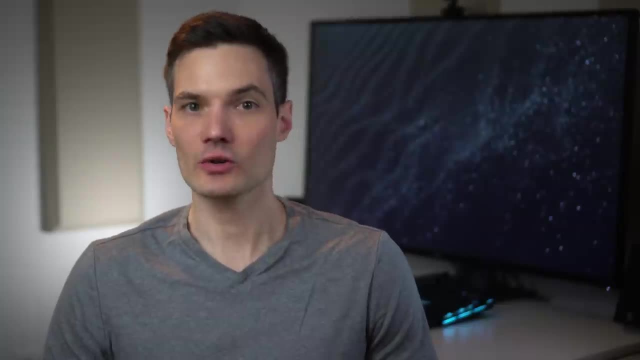 vivid and also appealing. You can also upscale the resolution and quality quality of the videos, even if the original was blurry or low quality. You could even add cool effects, and this one's really fun. You can put in transitions or 3D cartoons, manga pop and so much. 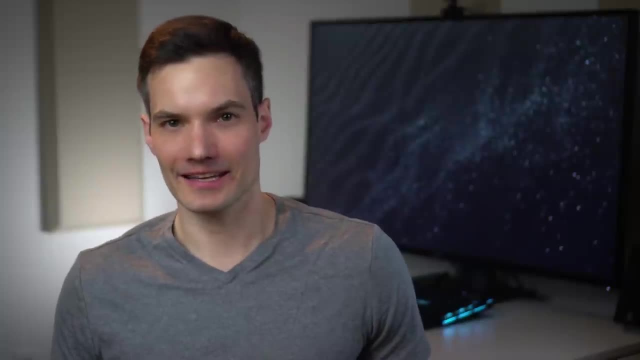 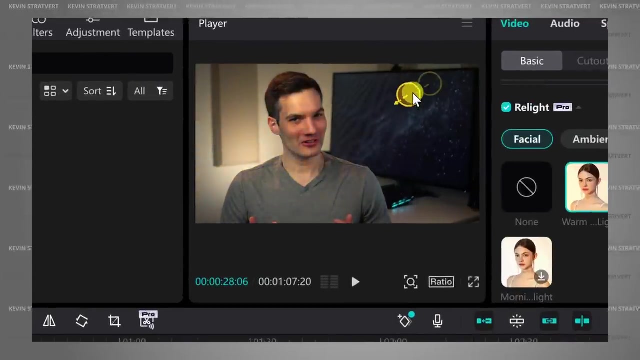 more. You can also relight a scene. Maybe your lighting wasn't ideal when you first filmed. You could position the light exactly where you want it and look at how it interacts with the person. It's kind of like having a 3D object in a scene You can also reframe Here. I have a video. 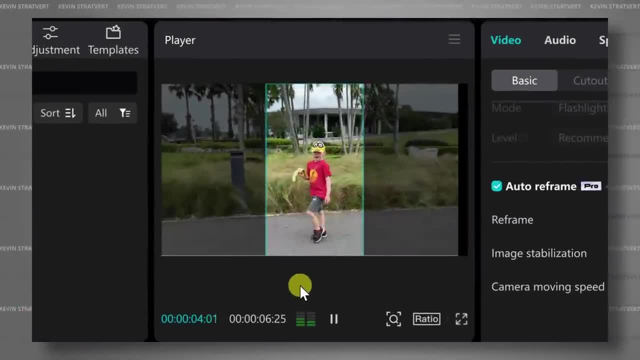 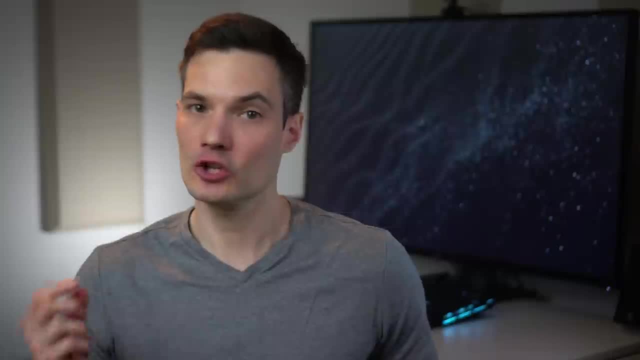 filmed in landscape, but when I click on reframe, it automatically detects where the subject is and then it locks on that. in vertical form. You can even refine the way you look using AI, For example. I can smooth out my skin or whiten my teeth, and there are so many other improvements and 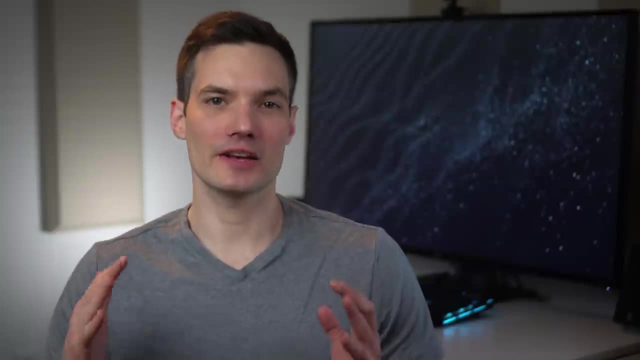 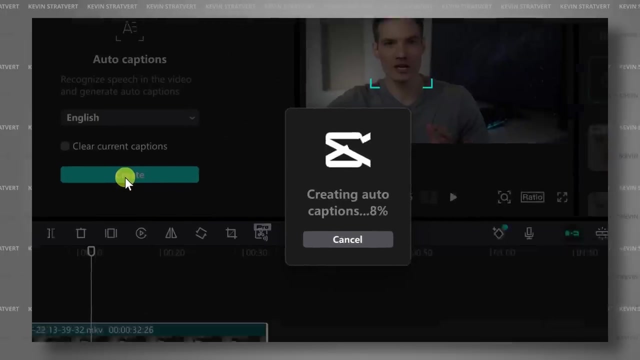 boy, I could sure use some of them. CapCut also has a number of AI tools to enhance the audio of your project. You can automatically generate captions from audio and it'll even style them forward and backward. You can also change the color of your image. You can change the color of your. 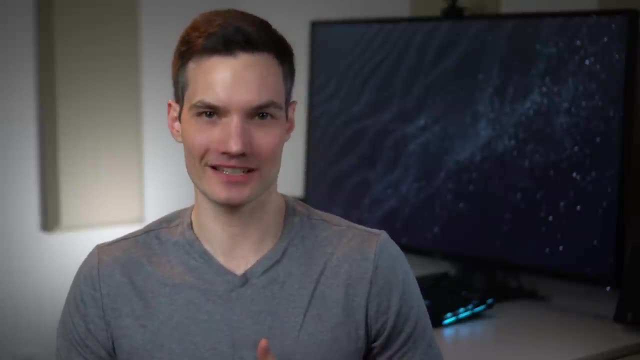 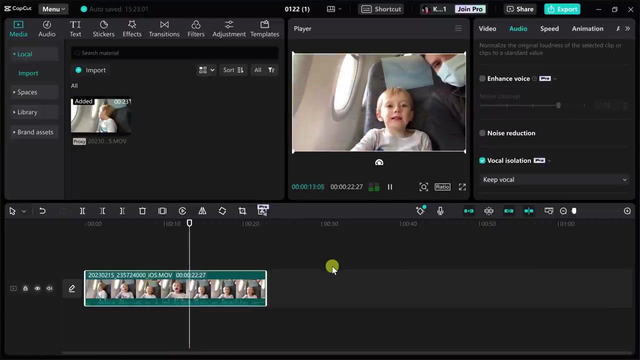 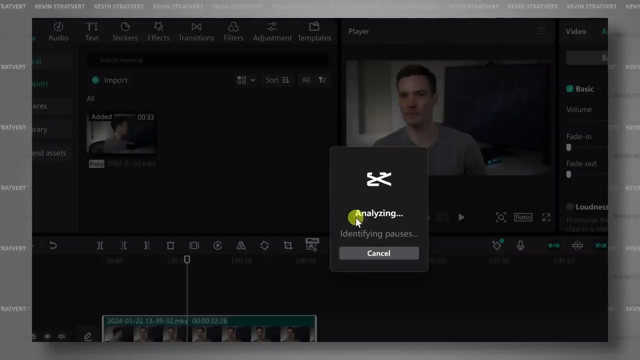 voice. You can enhance a voice and isolate a voice. Here's a video of me speaking on an airplane with lots of background noise. When I turn on voice isolation, it automatically removes all of that background noise. It's really kind of like magic. You can also improve how you speak by 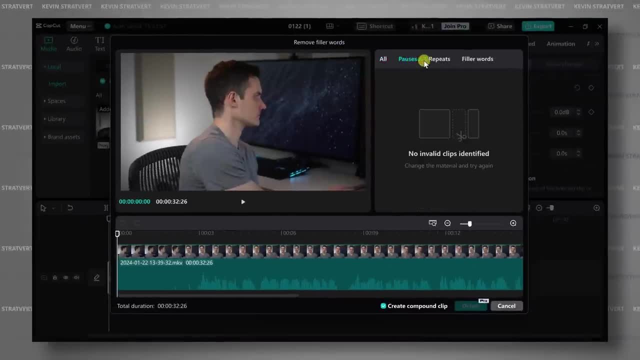 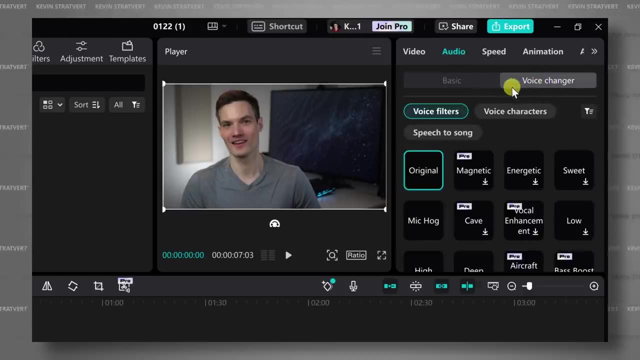 having AI identify and then remove all of those annoying filler words like um and ah- And this one is one of my favorites. You can also just change your voice into another voice. For example, I can speak as a werewolf and I can even set it to a song. 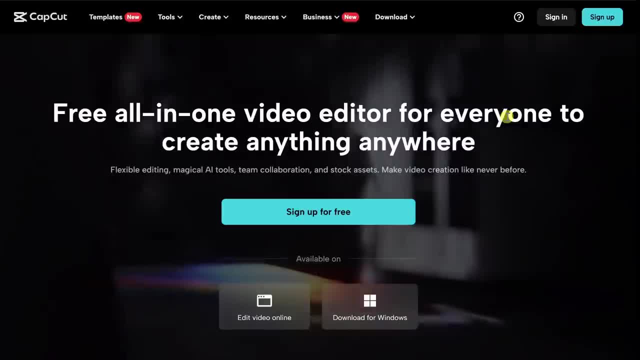 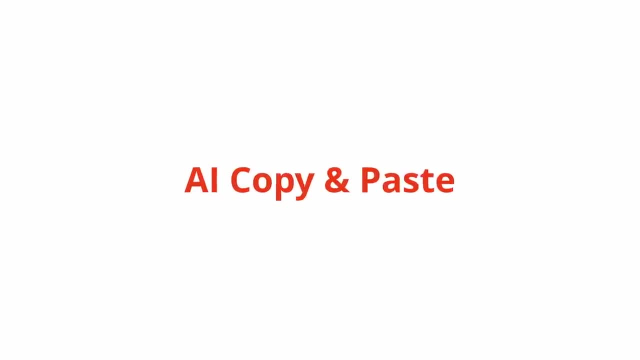 To get CapCut, head to the website in the description down below and then you can install it on your PC, or you could even use it directly on the web. Next up, we have UiPath Clipboard AI, If you spend any amount of time. 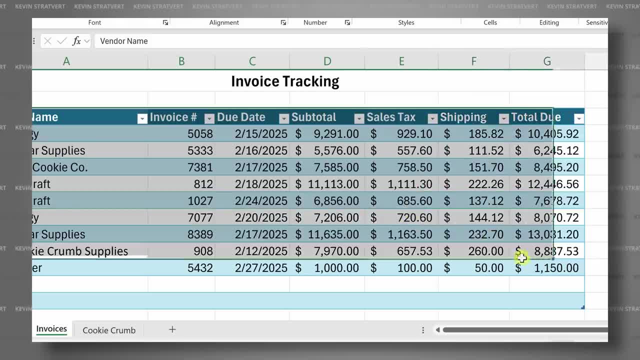 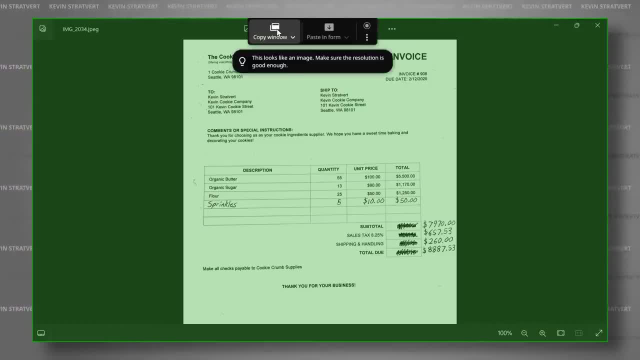 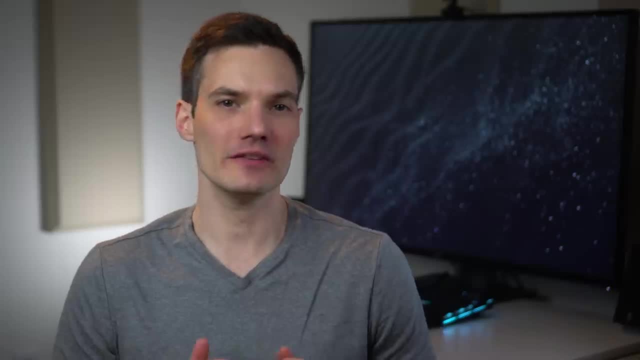 copying and pasting data from one application to another. you'll want to use this Here. I have an image of data that I need to get into Excel. I'll copy this using Clipboard AI and then paste it into Excel and it pastes all of the details, even the handwriting. You can even 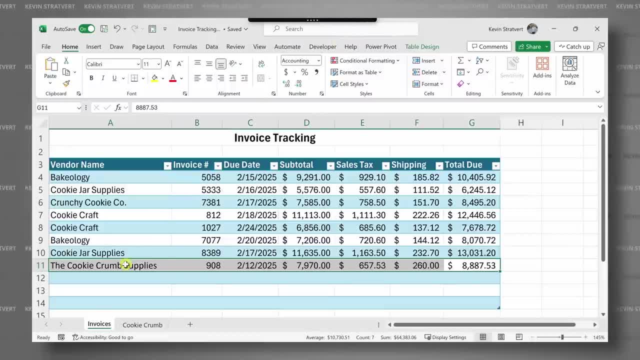 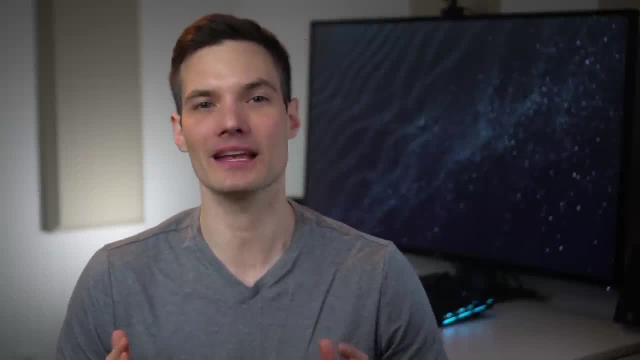 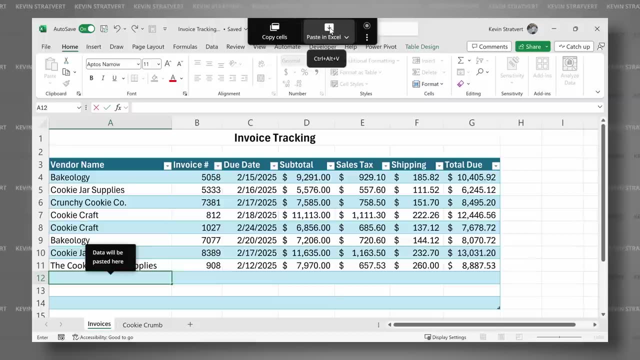 paste it into a pre-formatted table and it pastes all the data into the correct columns. This is an insane time saver, especially if you routinely copy and paste lots of data between applications. Not only that, but you can also copy a text-based message and it'll understand. 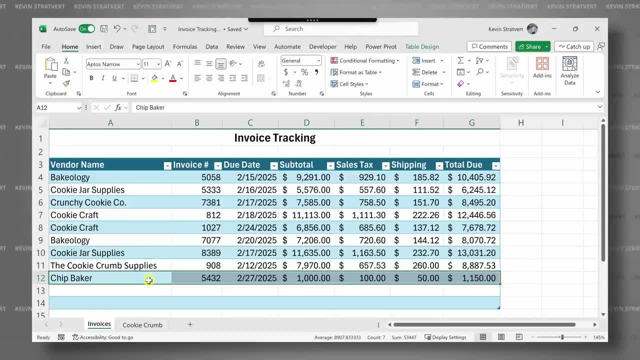 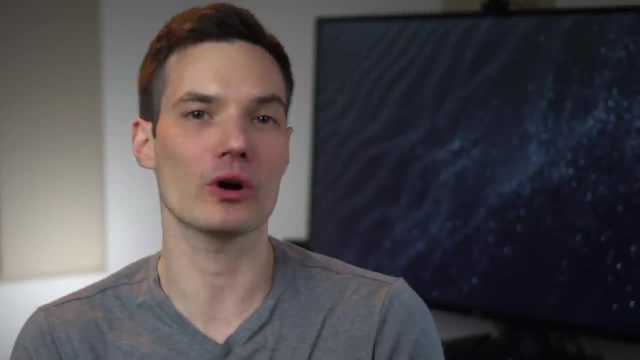 all the data from within the message and then you can paste that into the correct columns too. My mind is blown: You could even use it to copy a table of data in Excel and then use it to paste into a web form. If you do any type of boring copying and pasting, 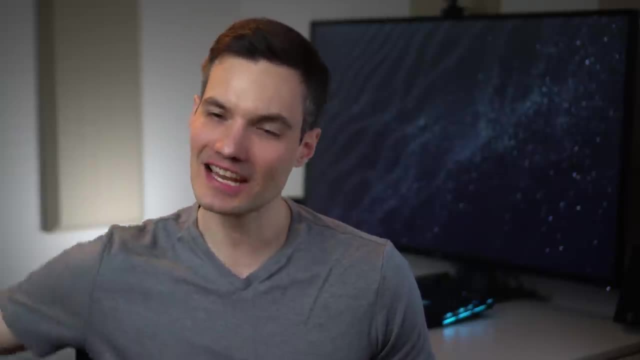 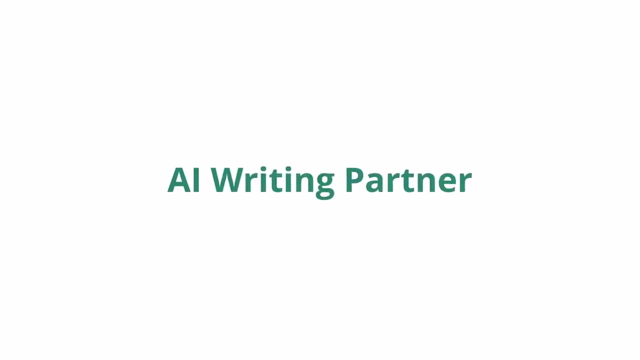 this is kind of like having your own personal wizard that can save you from all of that. To get this free tool, head to the website. in the description Next up, we have Grammarly, an AI tool that can help you with all parts of your writing. 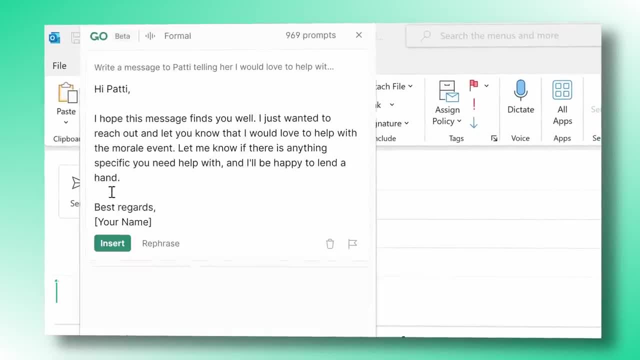 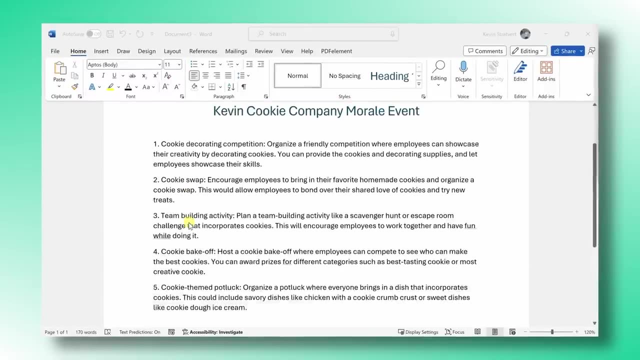 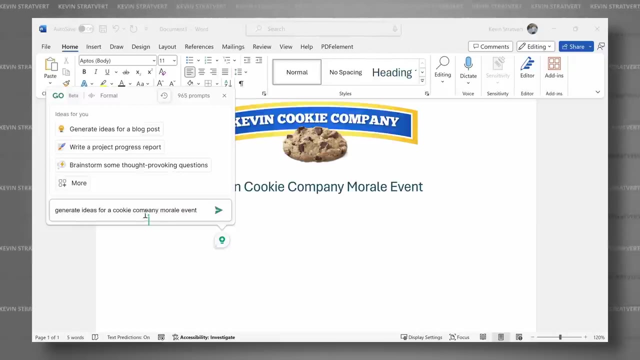 You can use it to brainstorm new topics, outline ideas, revise your writing and even polish it. It's like having your own personal proofreader and editor follow you around every time you write Here. for example, I need to write an invitation to a company party. I can ask Grammarly to. 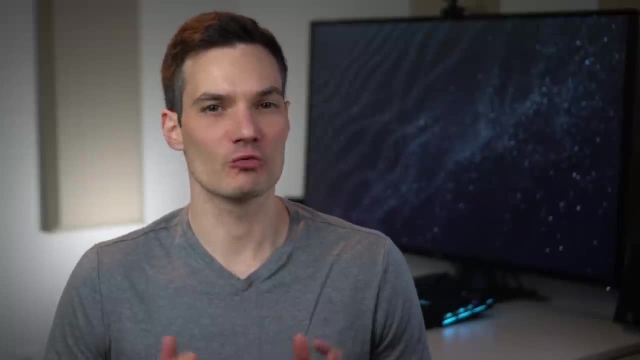 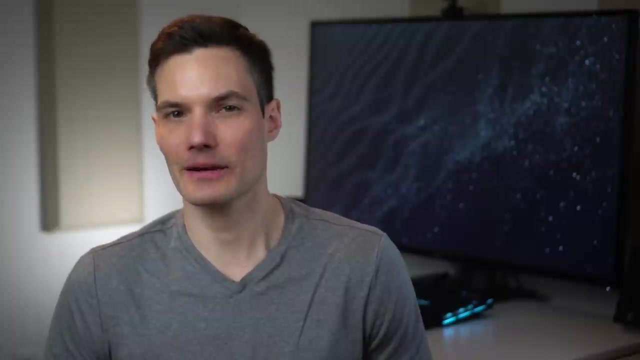 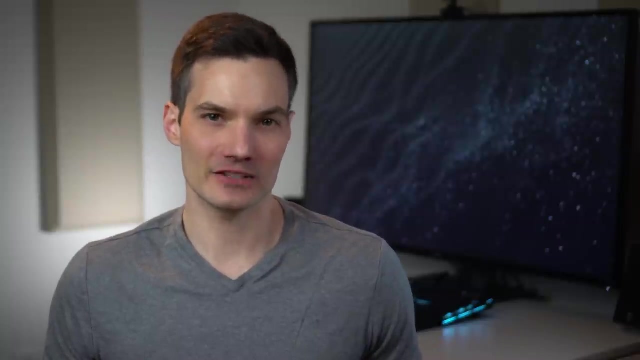 assist me with this. I can even use Grammarly to refine the message, Like: let's make the invitation a little more fun and maybe a little bit more humorous. As I type, I also get real-time suggestions with improvements to uplevel my writing. The thing I love about Grammarly is: 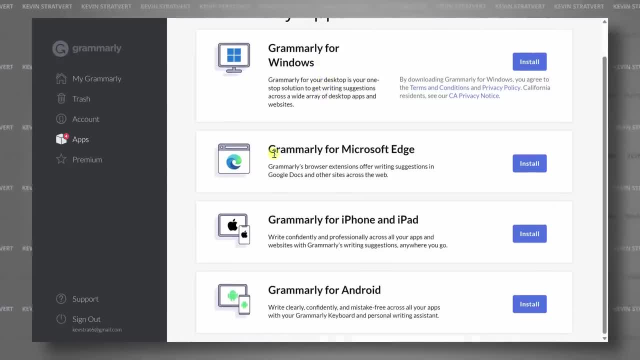 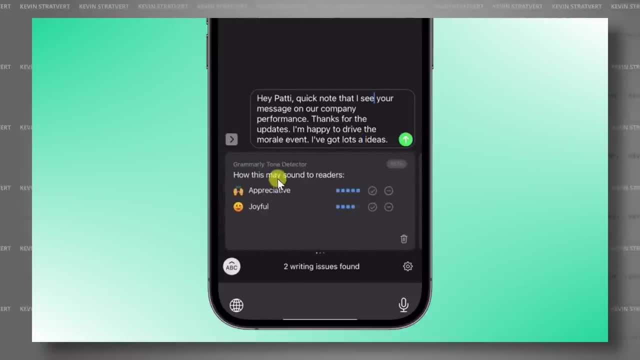 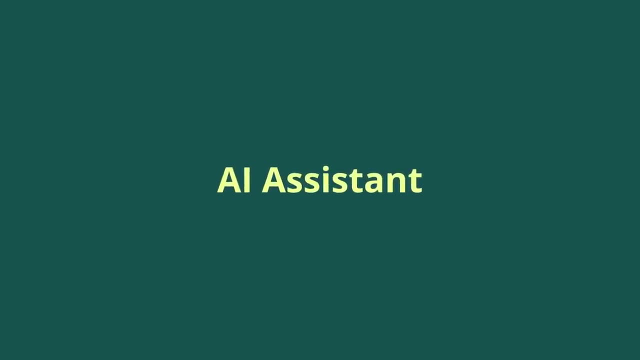 you can use it in any of the tools or places where you happen to work, like on Windows or Mac, in apps like Word or PowerPoint, or even on websites. You could also use it on iOS or even on your Android phone. Next up, we have OpenAI's ChatGPT, and it can help you with just about anything. 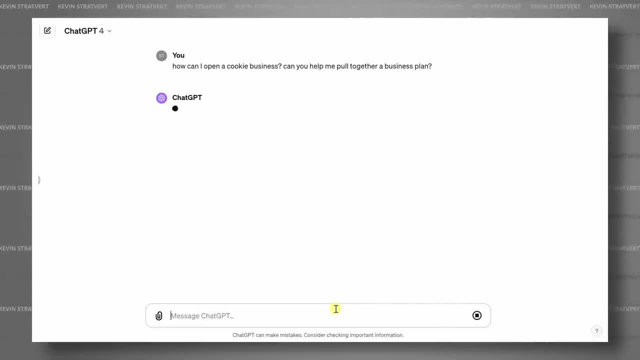 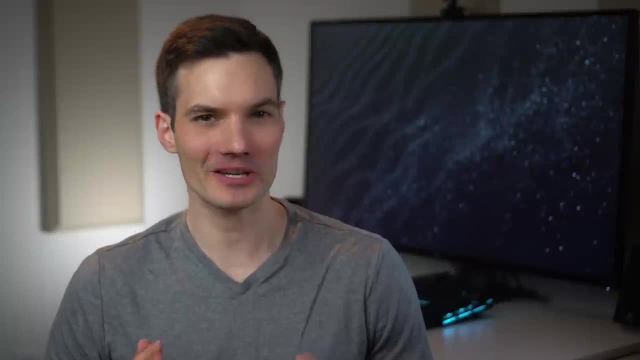 At a very basic level. ChatGPT is your AI assistant. You can ask it a question, get an opinion or even ask it to code or analyze data, and it does a pretty darn good job. For example, write a short song about the Kevin Cookie company Nice. 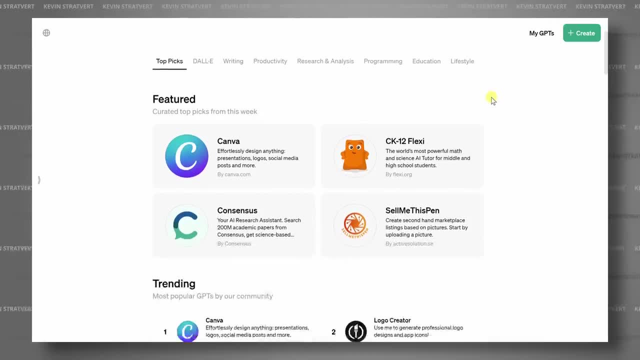 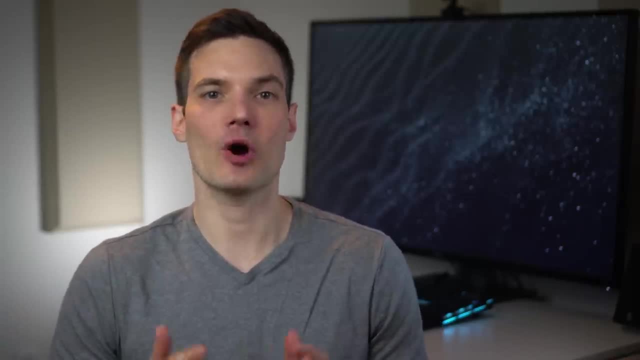 More recently, you can now access something called the GPT Store, which extends the power of ChatGPT as long as you have a premium membership. For example, here's an app called ConsenSys and it'll analyze thousands of peer-reviewed 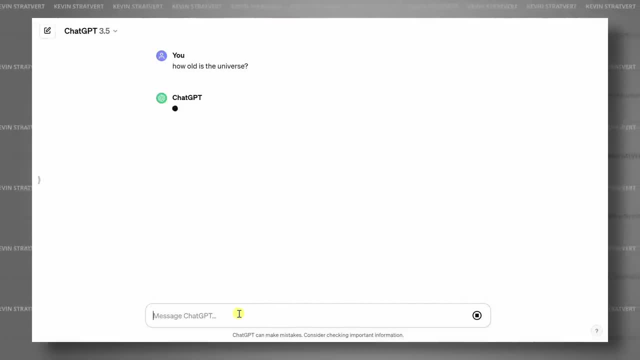 and also published papers. For example, how old is the universe? You can also get access to something called the Data Analyst Here. I'll drop in an Excel file and it'll analyze it for me. Look at those interesting insights. I could even ask it. 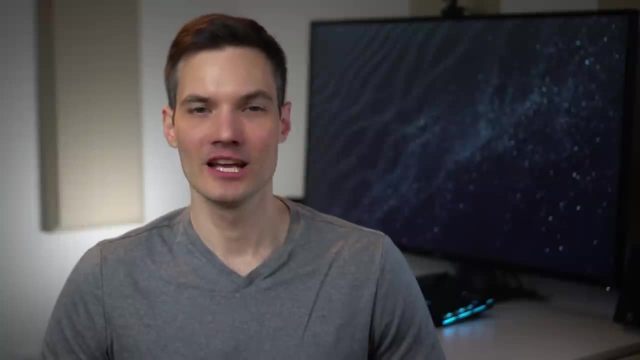 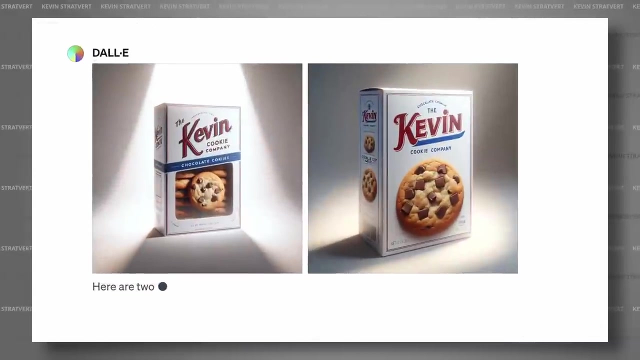 questions. That's so valuable and also easy. You can also use ChatGPT to generate images like: make a product shot of a box of Kevin Cookie company chocolate chip cookies. Ooh, that looks good. We'll use that on our website. 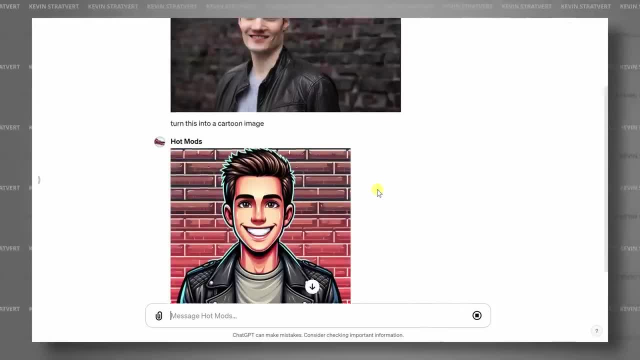 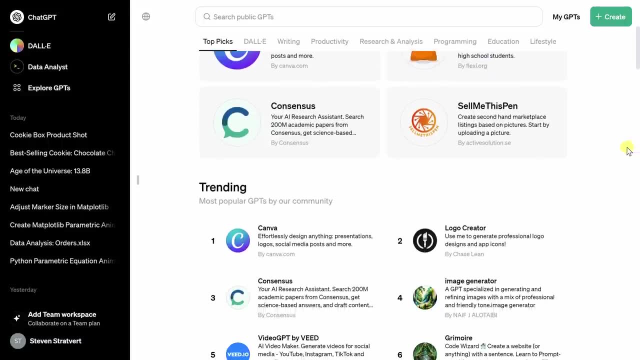 You can even turn a photo of yourself into a cartoon image. These are just a few examples of what you can do. You can get ChatGPT at the website in the description down below, And if you want some more advanced features, you'll have to go premium.